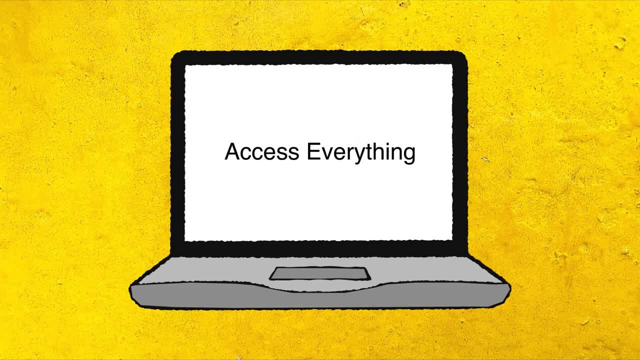 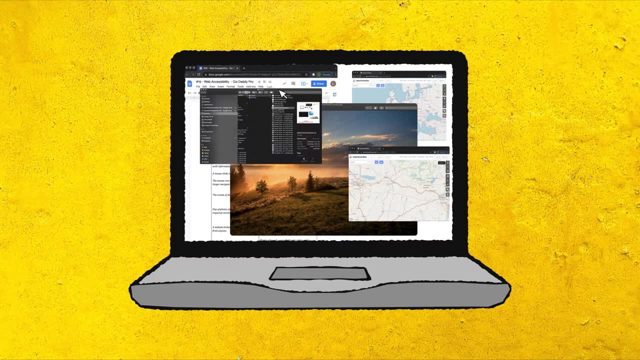 It can be hard not to think of the web as a great equalizer, One that has granted unparalleled access to a treasure trove of information and connections to all who log on. Imagine, if you can, that you can't use a keyboard or mouse to 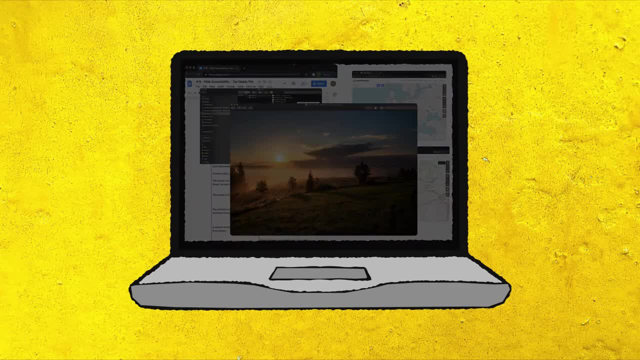 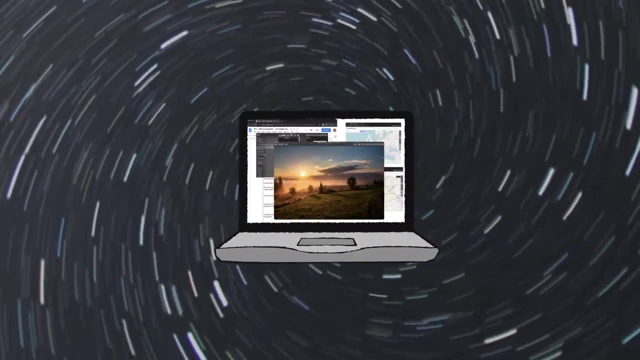 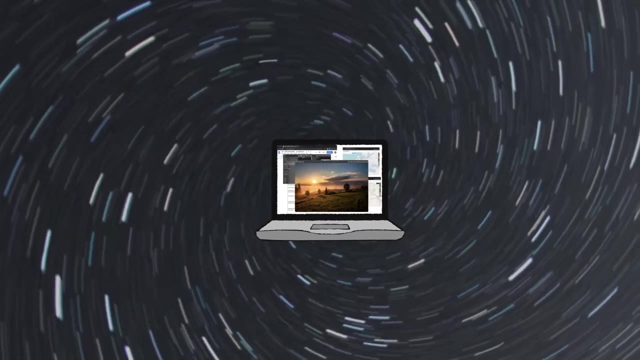 navigate. Now turn off your screen and try to get to a new website. These are the challenges the visually impaired and individuals with severe tremors or paralysis face when it comes to accessing the web. in a way, most of us take for granted. From that perspective, the world wide 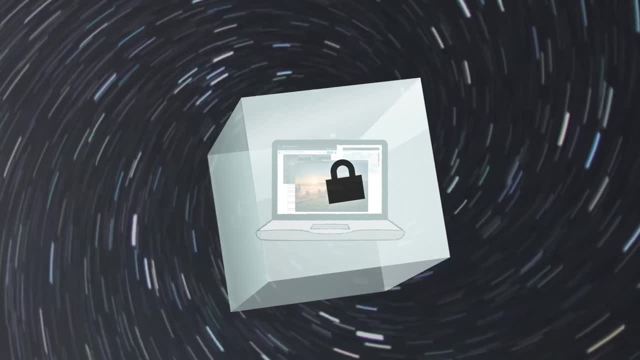 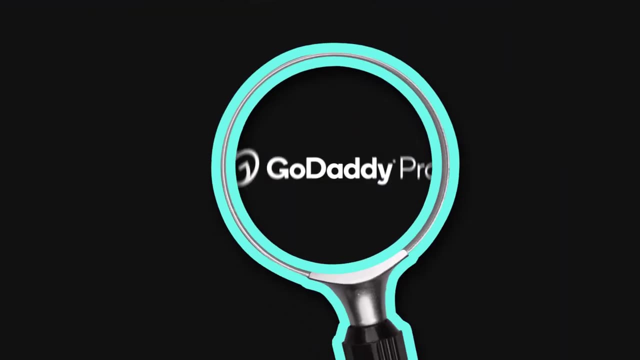 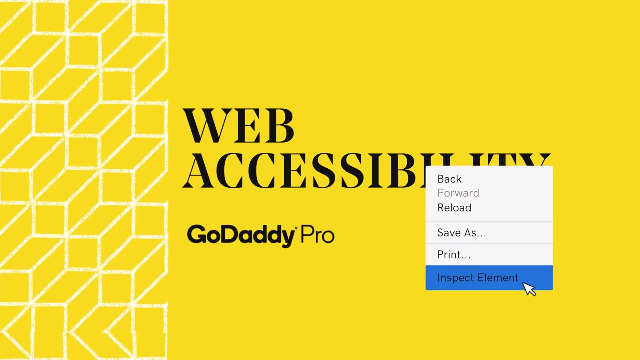 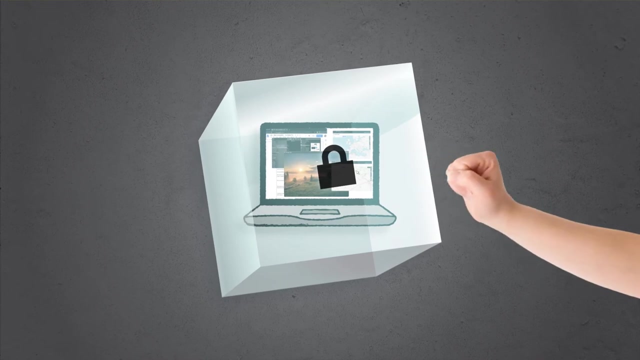 web doesn't seem so free and accessible. That's why web accessibility should be at the forefront of any choices we make when designing and developing websites. Web accessibility: Web accessibility is a. Web accessibility is a about breaking down barriers that prevent visitors from interacting with the content of a website. 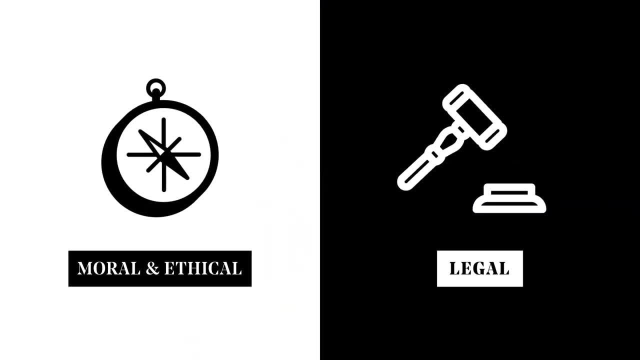 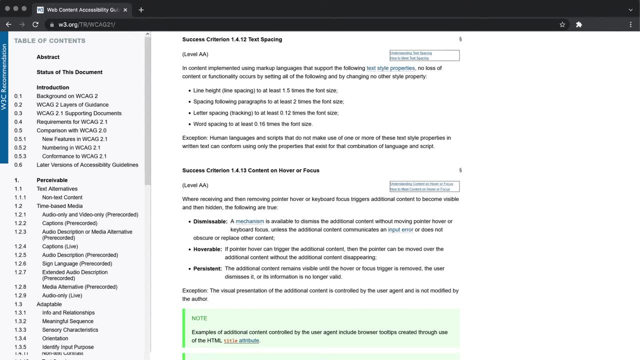 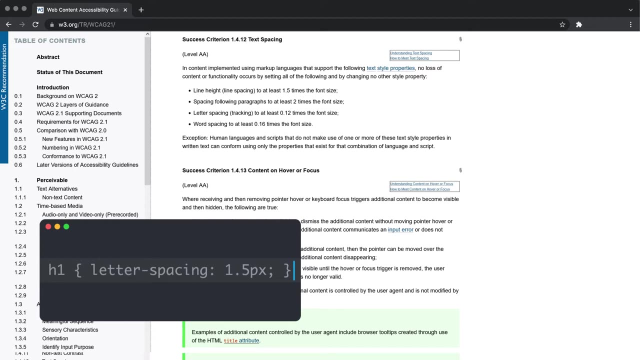 There are moral, ethical and legal reasons to make websites more accessible. No matter the reason, you can accomplish this by following defined guidelines when coding a site, That's it. In many cases, a few characters or words of code in the right place will do the trick. 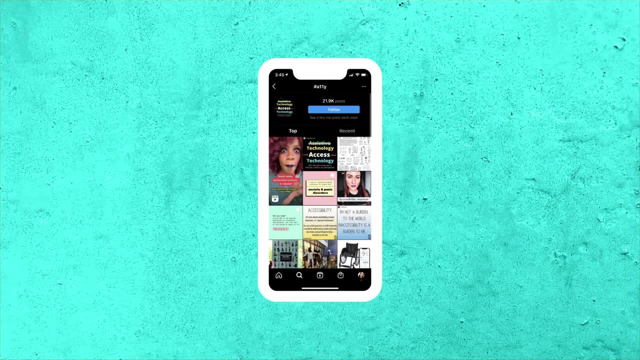 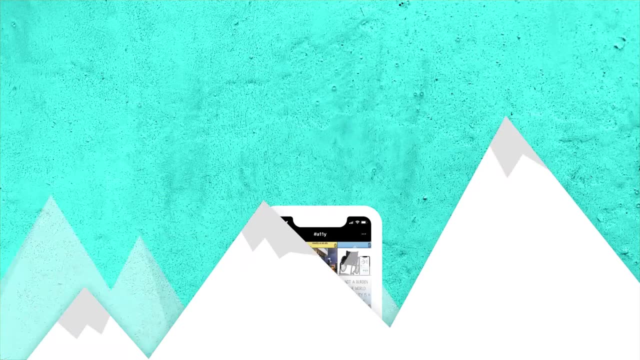 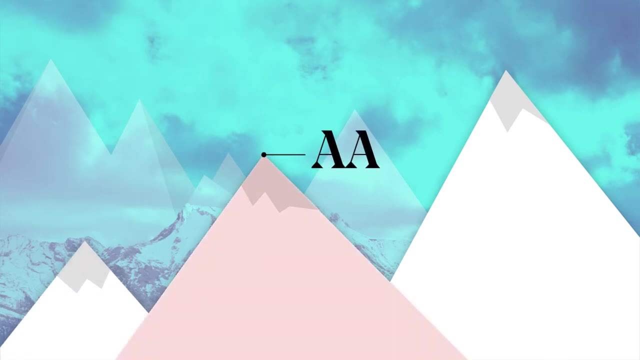 You can see the important conversations happening around accessibility led by the accessibility community by searching for the A11y hashtag on Twitter and other social media. There are three levels when measuring accessibility: A, which is the bare minimum. Double A is the target level for many businesses. 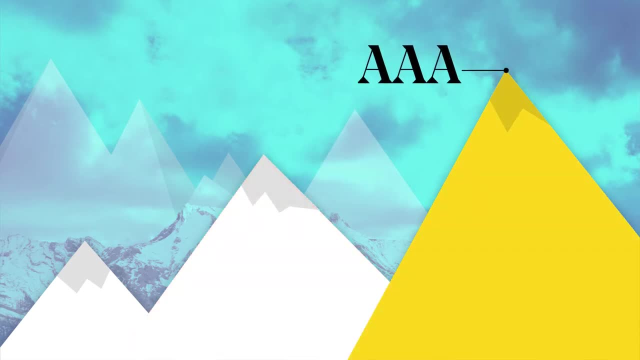 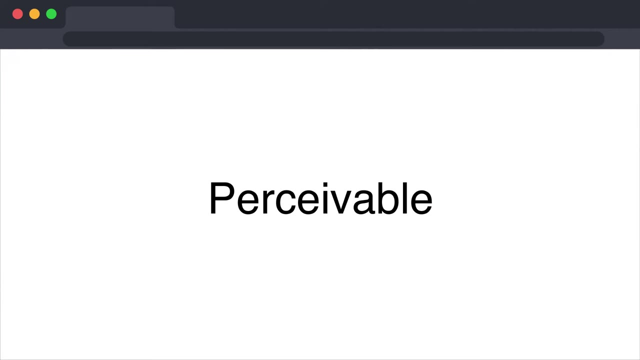 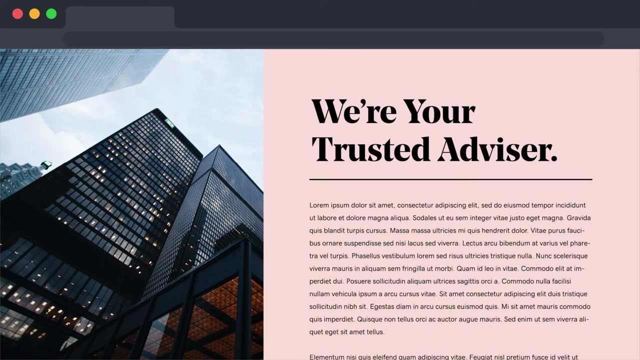 And triple A is typically reserved for special dedicated software. The guidelines are organized around four principles: Perceivable Information and user interface components must be presentable to users in ways they can perceive. This includes standards such as providing text alternatives for non-text content. 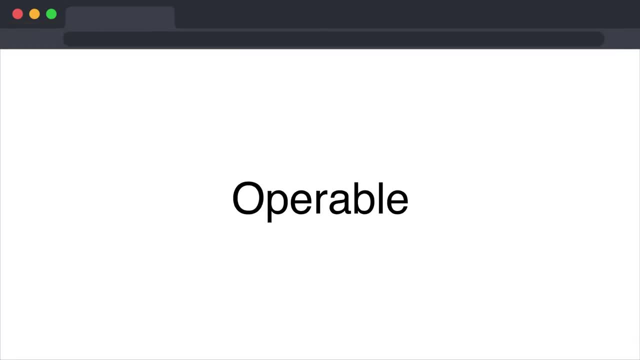 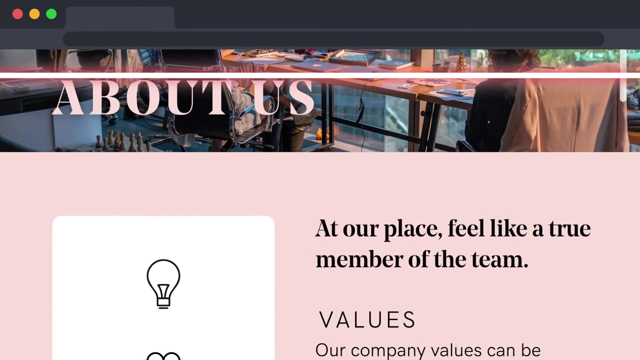 Operable User interface. components and navigation must be operable. For example, all functionality must be available from the keyboard. Understandable Information and the operation of user interfaces must be understandable. This includes, for example, a requirement to identify the primary language of the page. 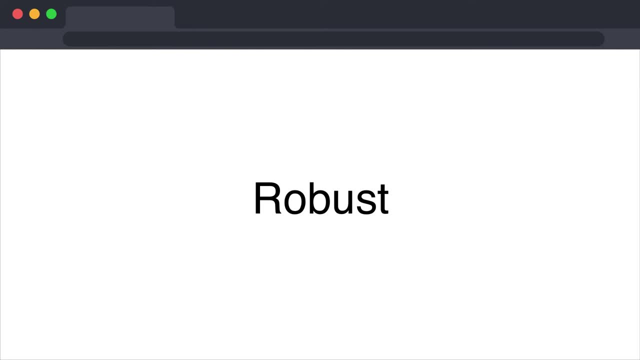 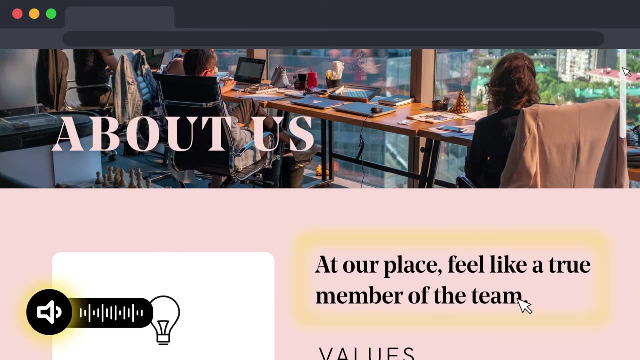 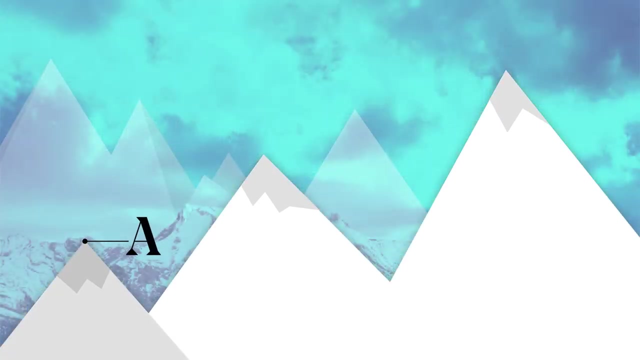 Robust, Understandable. Understandable Content must be robust enough that it can be interpreted reliably by a wide variety of user agents, including assistive technologies. This means being certain to use valid markup. for example, Conforming with level A brings basic compliance to your site. 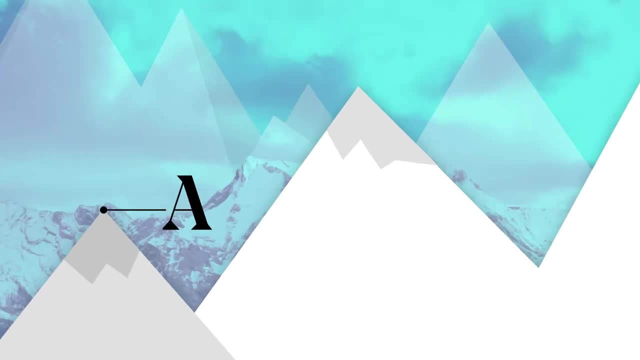 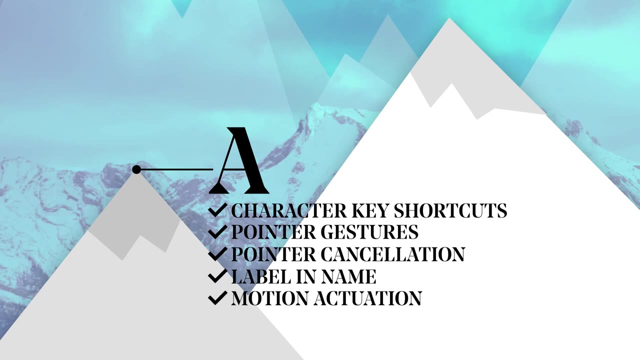 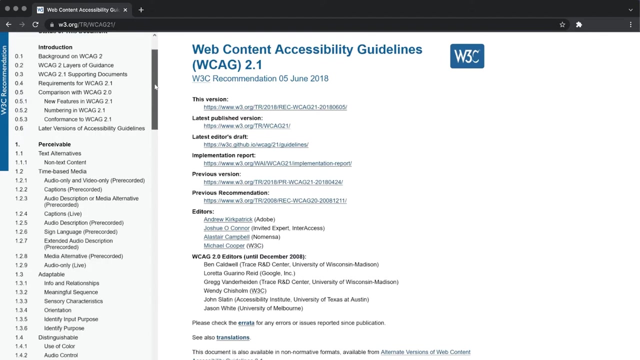 With each level you step up, the more accessible your site becomes. Hitting the basics of web accessibility is relatively easy, although it becomes more complex when you dive deeper into issues and solutions, Even if you can't get full WCAG 2.1 compliance right away. 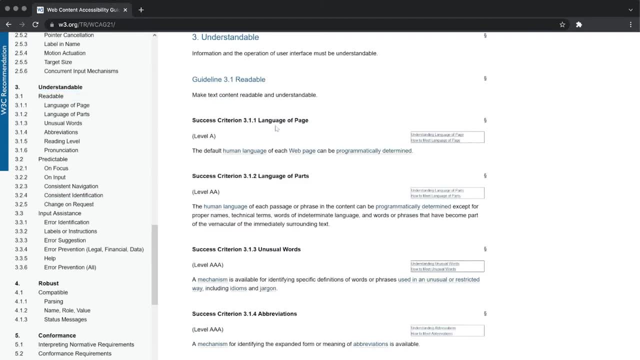 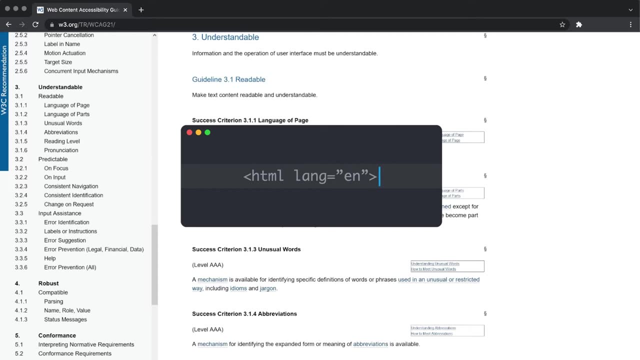 there's still plenty you can do to make a website more accessible, Like help screen readers identify the primary language used in the document, which you can do in HTML. Every page title should adequately and briefly describe the content of the page, meaning each page has. 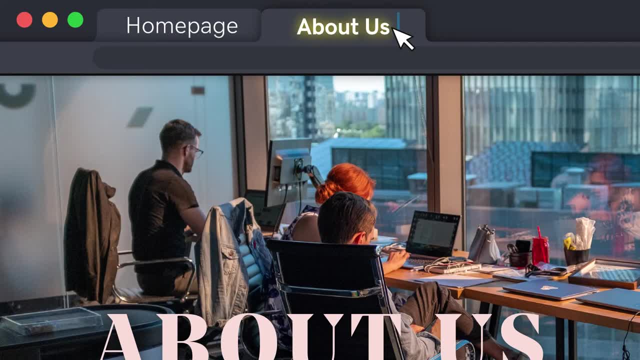 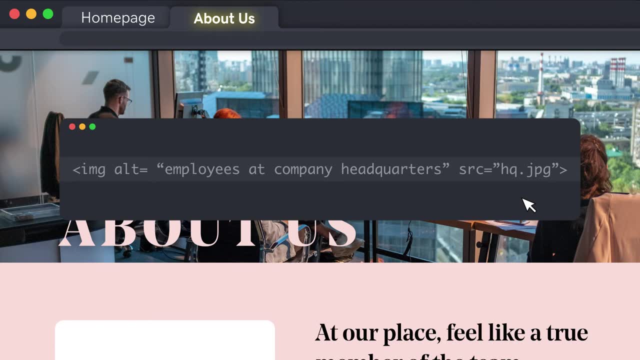 a unique title that distinguishes it from other pages. Make sure all images include equivalent alternative text, So the pick of your company has to be consistent. This is the most common example of this, because the performance is very limited, but you can still improve your site's accessibility. 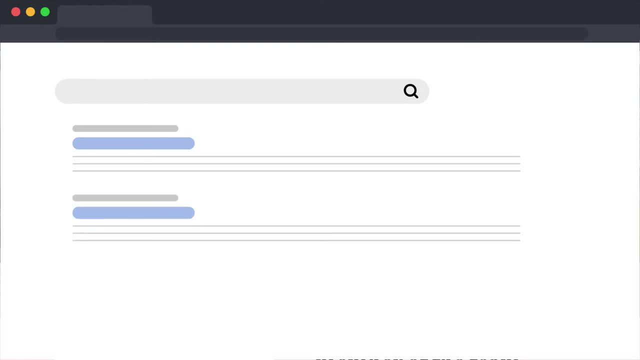 There's great variety of options for right to left, For instance, using the Whiteboard on the right side of your image should be no problem in using the Whiteboard. however, the same works for the other side, Using it on all pages. 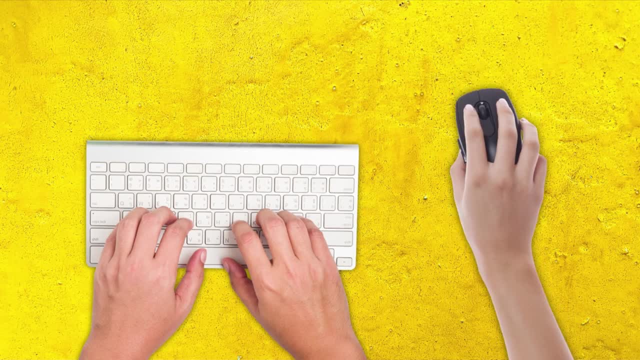 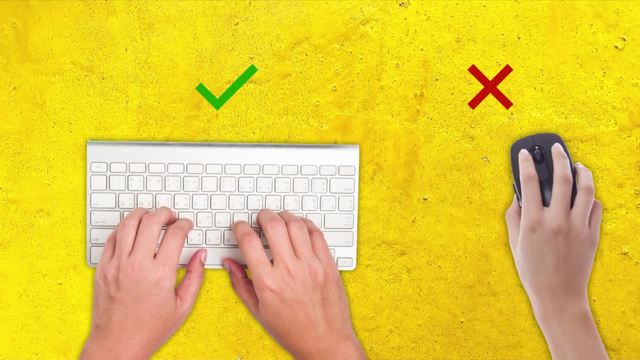 but with different options is definitely easier. Without the alt, the image doesn't exist for a visually impaired visitor, search engines or people who have turned off images. Everything should be workable from a keyboard, as many people cannot use a mouse. your audio file is likely inaccessible to people. 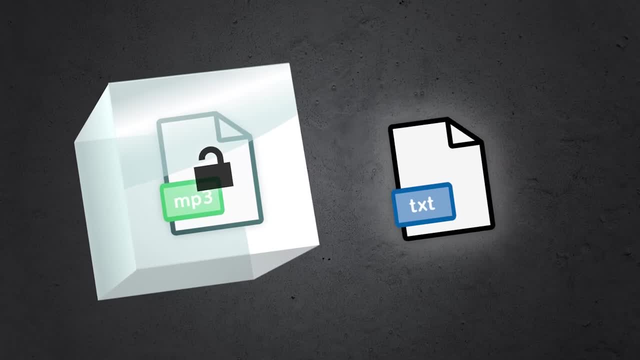 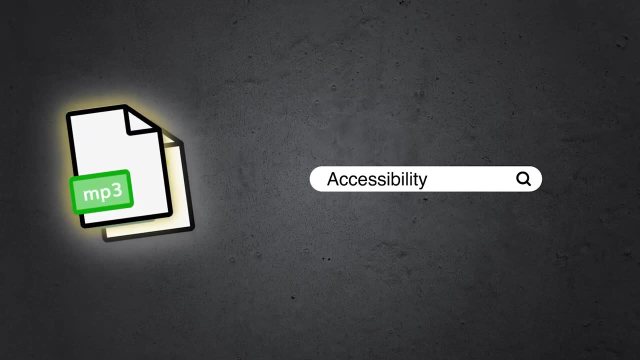 who are deaf or hard of hearing. As an added plus, your transcript will be searchable and add to your SEO. You can even use a transcription service if you don't wanna do it yourself. Users should be able to determine the purpose of the link. 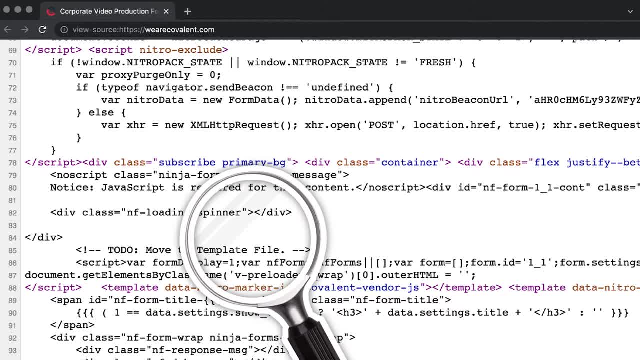 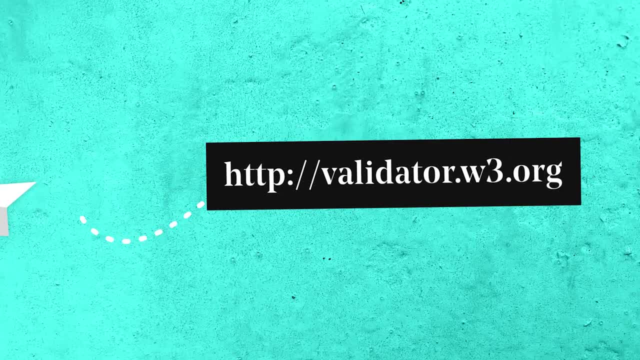 from the link alone and or its context. Missing open or closure brackets can really mess up a screen reader, so be sure your pages are properly formatted. You can use this markup validation check to find potential errors. As a person working in the space, 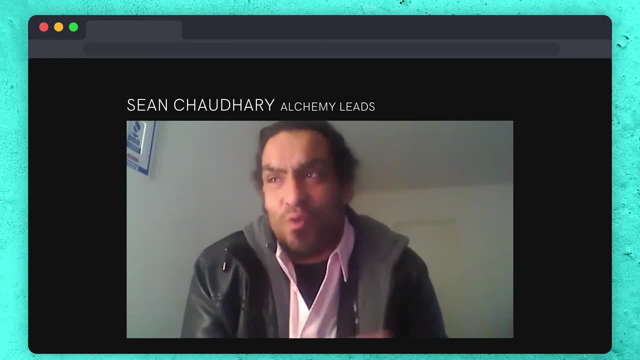 it's easy to complicate things, and as well you can get lost in the legalese. Whenever you get down to legal things, it can seem more complex than it really is. so I say keep it simple. The simple way to put it is just experience, or accessibility. 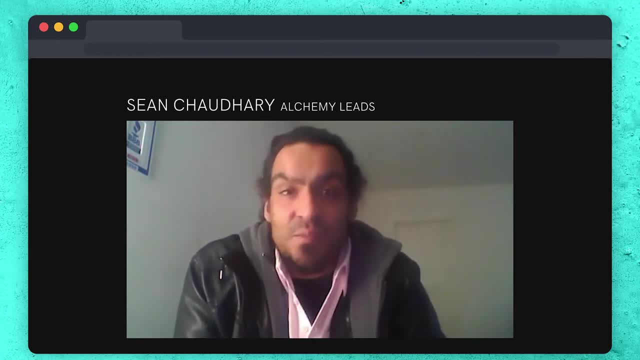 I can define it in literally one sentence: text behind visual elements. Once you know that you can pretty much do anything, You know the best way to do it, the most compliant way to do it, which is page titles. make sure you have them. 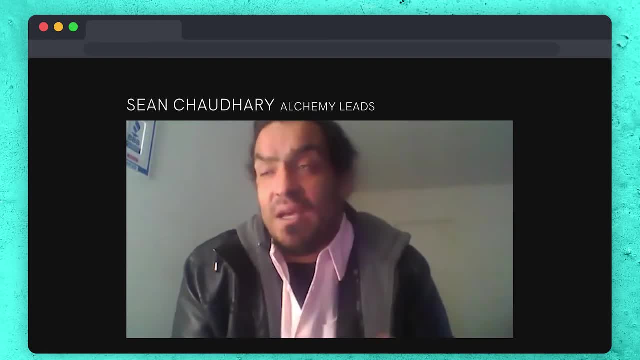 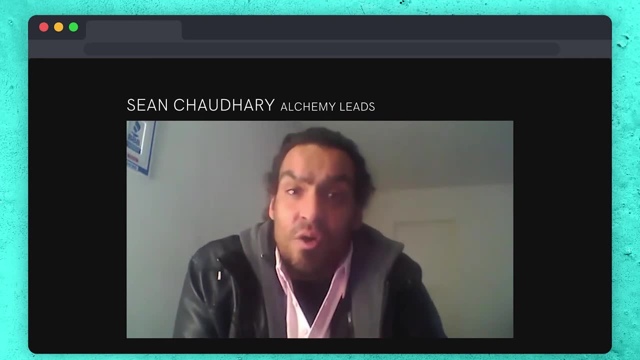 images, videos, right. So make sure your videos have subtitles. If not, you can even get them transcribed- There are also tools to do that- and have that somewhere on your page. And then images: make sure your alt tags are properly filled in. 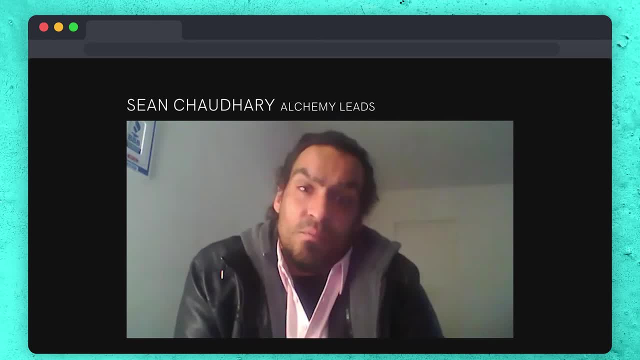 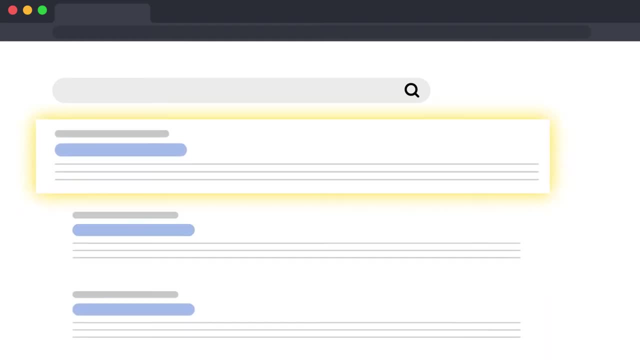 and you can even optimize them for SEO. But all of that relates back to just keeping it simple. Perhaps you'll notice that a lot of these items are also good for SEO, so you'll get a double bang for your buck on any accessibility work you do. 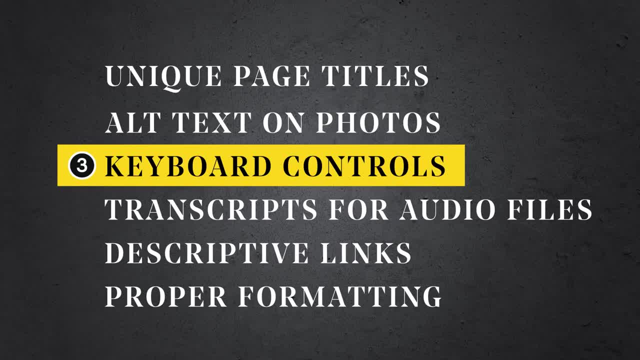 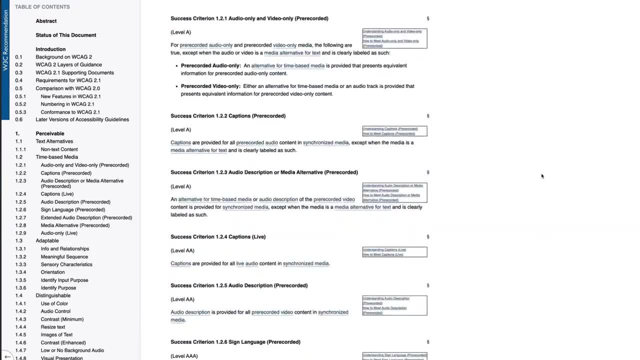 These steps are just the beginning, but they will greatly improve a site's accessibility with minimum work. You can check out the web content accessibility guidelines to see what else you can do. The tough thing about boosting accessibility is that there are a lot of rules to follow. 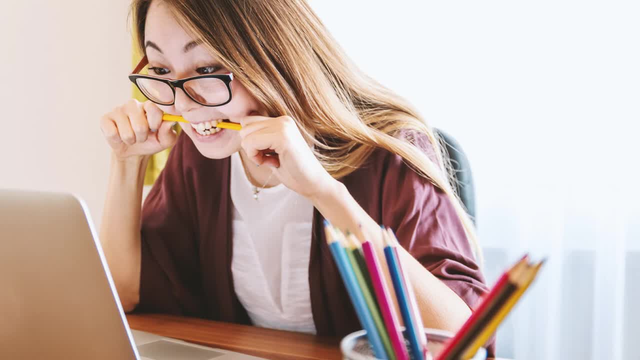 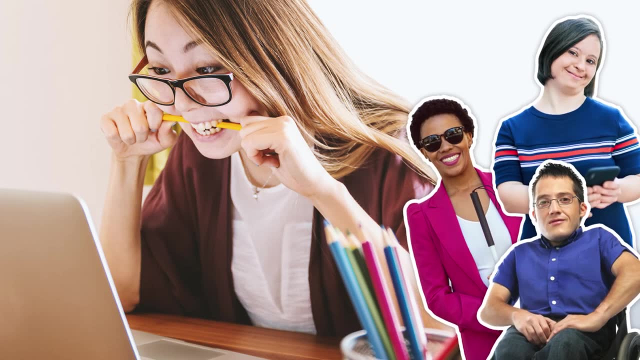 to lift your site up to a high accessibility level, especially if you're working with legacy code. However, even if you're never planning to make it all the way to WCAG AA compliance, you owe it to your users to take as many steps. 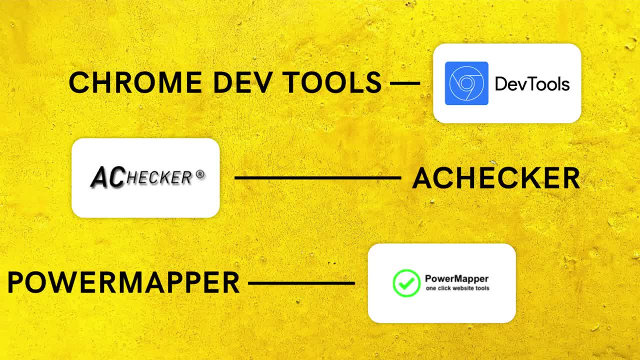 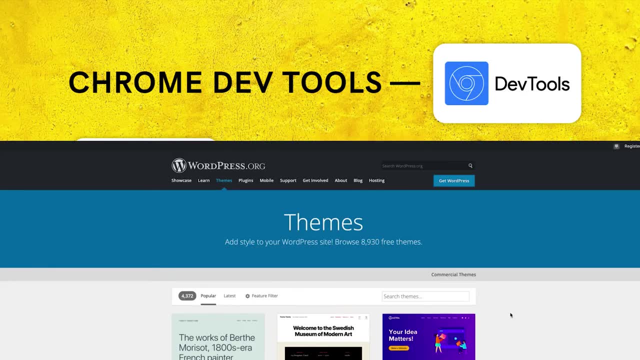 as feasible to make your content accessible. You can assess a site using accessibility assessment tools like Chrome, DevTools, A-Checker and PowerMapper. If you're a WordPress dev, you'll be happy to hear that, as of March 2016,, all new or updated code. 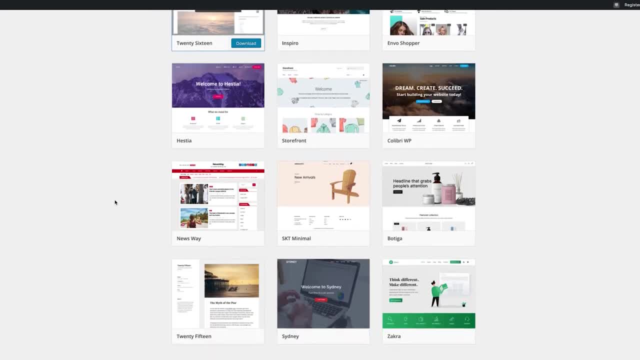 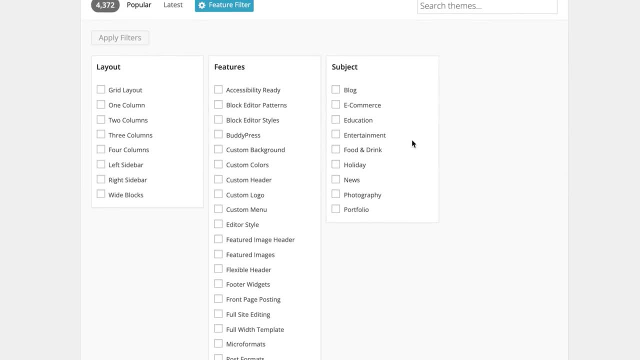 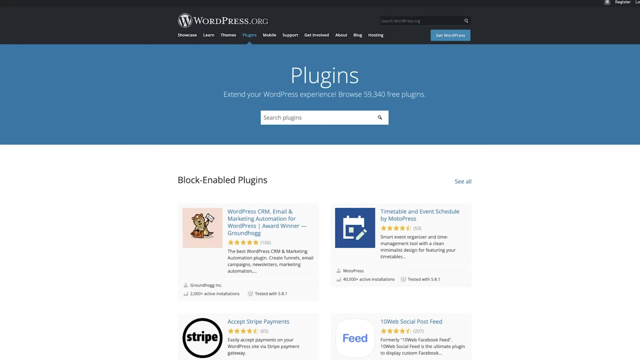 released into the WordPress core and bundled themes conforms to WCAG 2.0 guidelines at level AA. In the WordPress theme repository you can search for themes with the accessibility ready tag. The themes are another story, as they're not audited by anyone for accessibility.